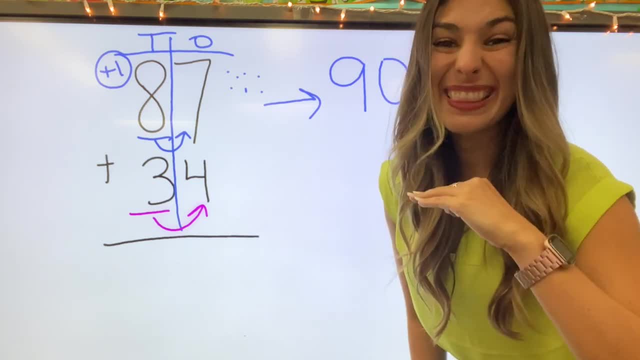 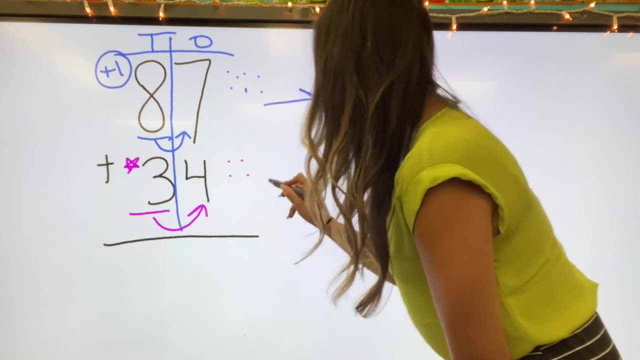 Five or greater, add one more. Four below, let it go. So four is less than five, So I'm gonna leave this three alone and bring it over here to 30.. So now that I've rounded both numbers, I'm ready to add. 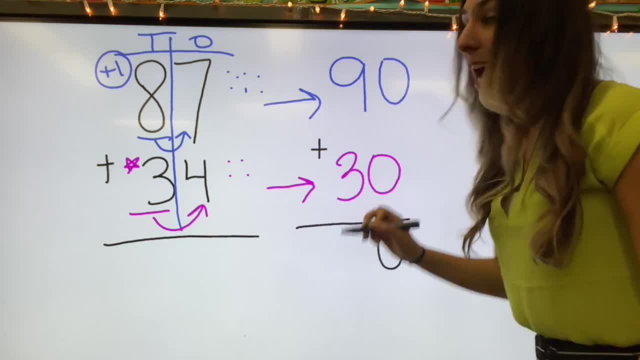 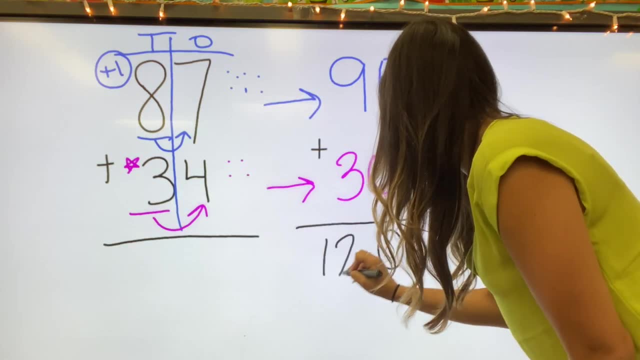 zero plus zero equals zero. nine plus three. I'm gonna put nine in my head, three on my fingers, Nine, ten, eleven, twelve. So my answer is 120, so let's go back over our steps. Let's review. So my answer is 120.. So let's go back over our steps. 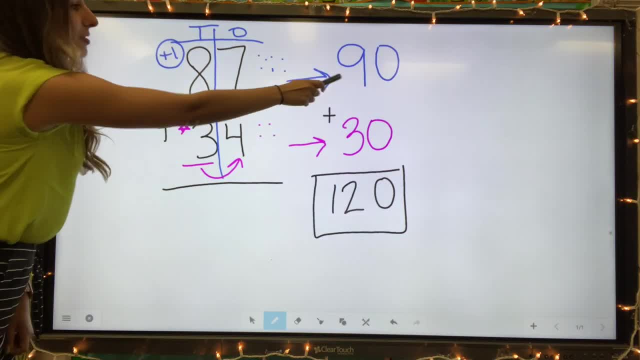 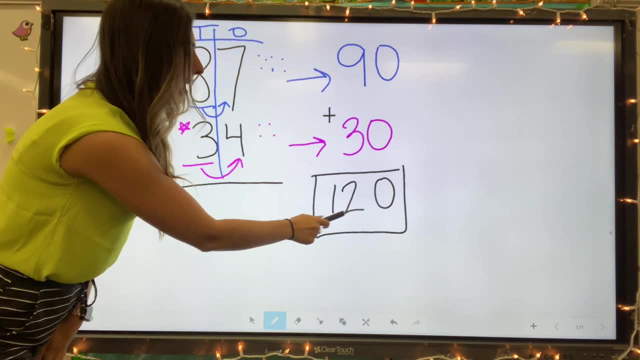 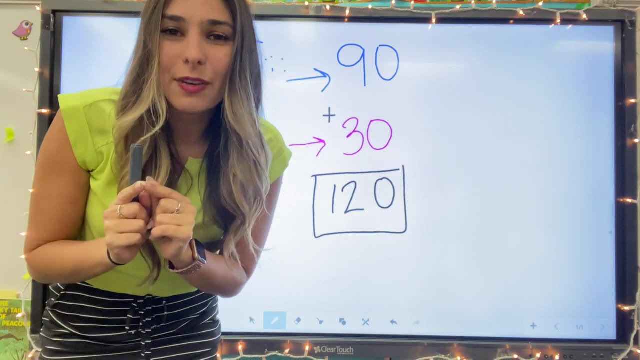 first, we rounded each number. the 87 goes to 90 and 34 rounded to 30. we added them up and found the estimated sum is 120.. now, when we estimate, it is not the exact number that this would add up to, but it's okay because we're looking for the estimate we're looking for about how many. so 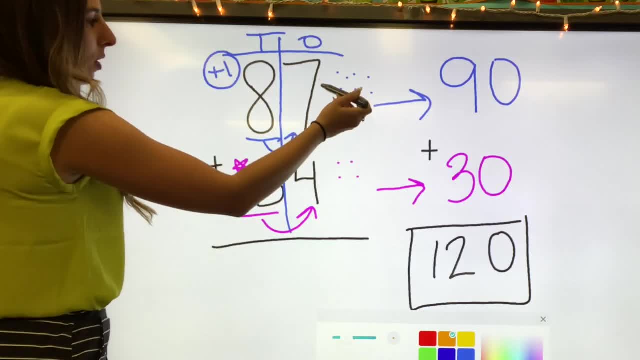 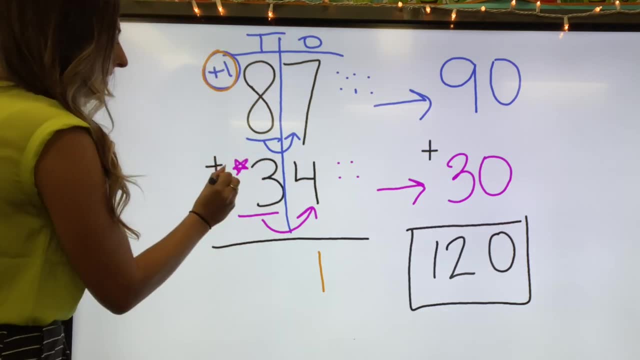 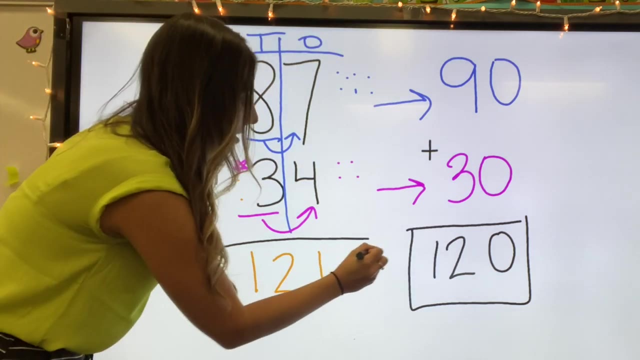 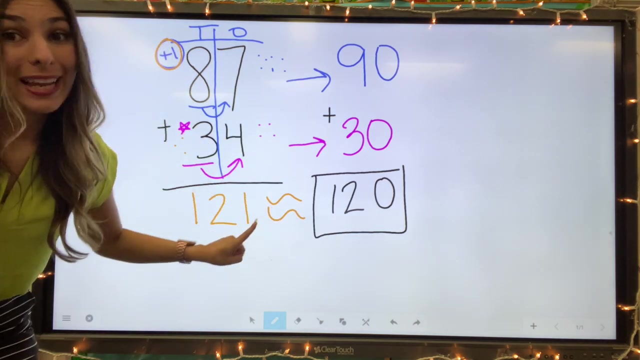 let's actually add this up and see if we were close, we would add ones first. so seven, eight, nine, ten, eleven, carry that one. we have eight, nine, ten, eleven, twelve. oh, so our real answer would be 121, which is about 120.. so our rounding and adding was correct, because this number is pretty dang. 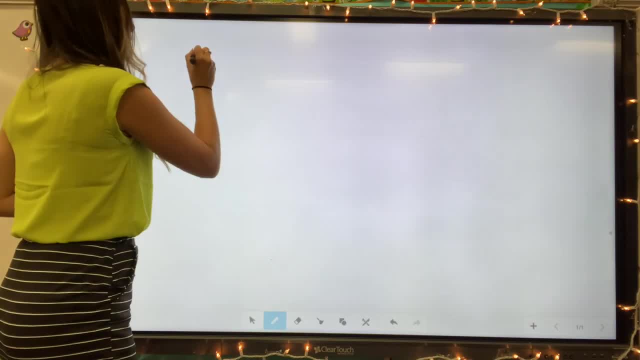 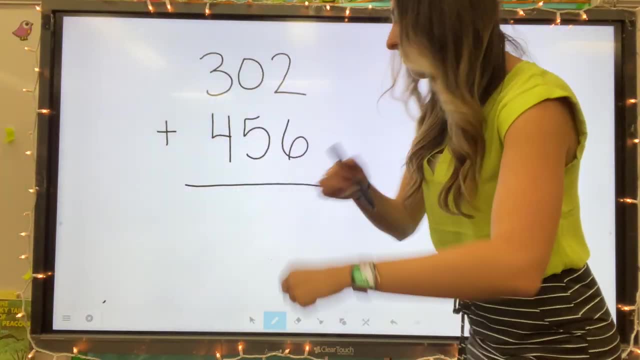 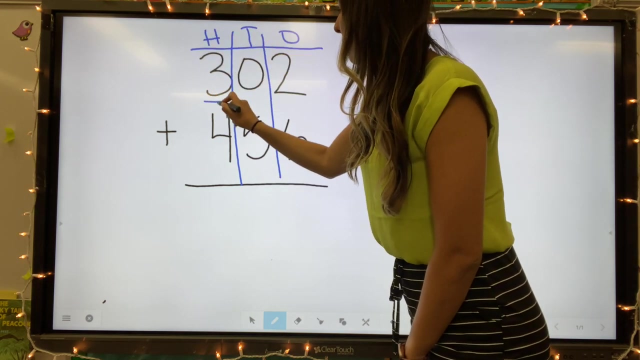 close to this one. all right, let's do a bigger problem. well, first thing i need to do is round each number. so to round, i'm going to follow my usual steps. my place is the three. i'm looking next door at that zero and i'm asking myself: five or a greater? 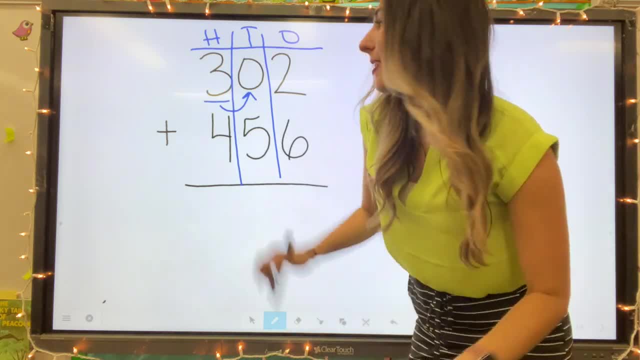 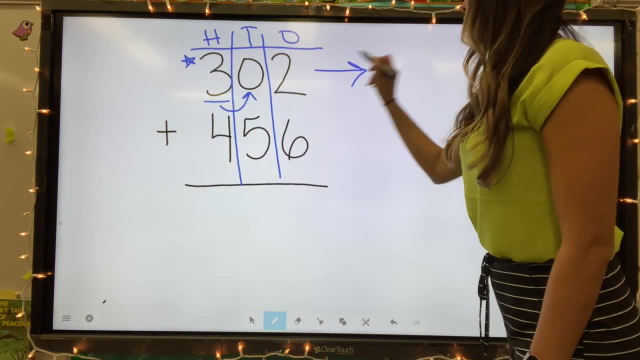 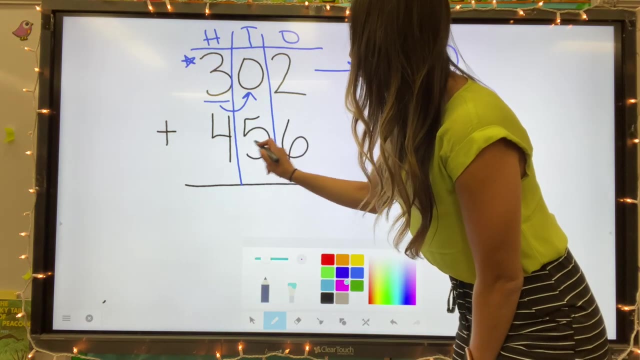 add one more four below. let it go that zero is way less than four, so we're gonna keep this three and round 302 to three. make that a hundred, three hundred. let's move on to our next number we have. My place is in the hundreds. I look next door at that five and I ask: 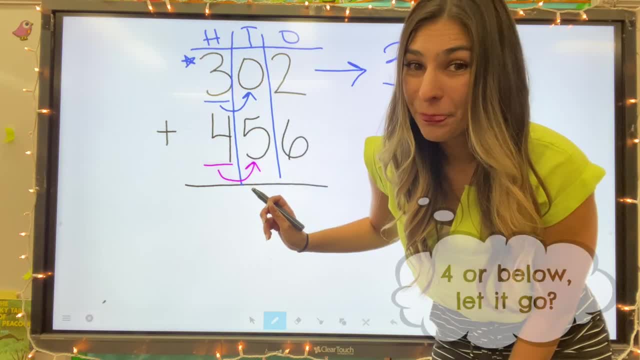 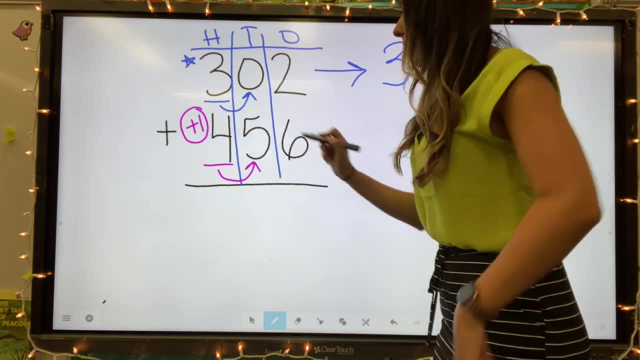 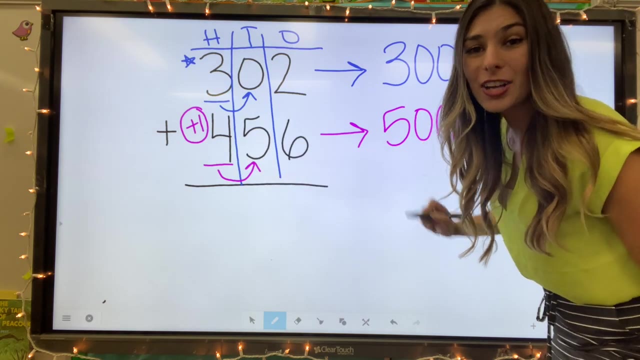 myself. should we add one more or let it go? We're gonna add one more. That five is too big. We're gonna add one more to our tenths. So four plus one equals five. We're gonna make it a hundred. So we rounded 456 to 500.. Now that we've 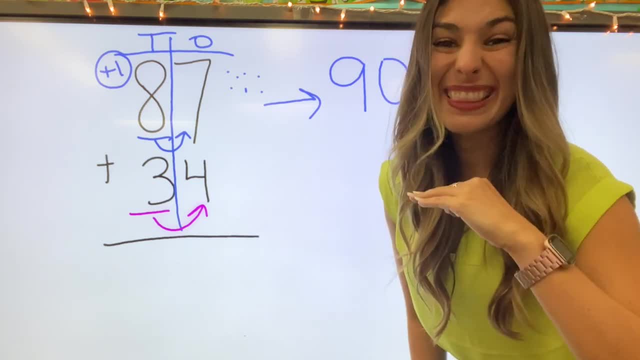 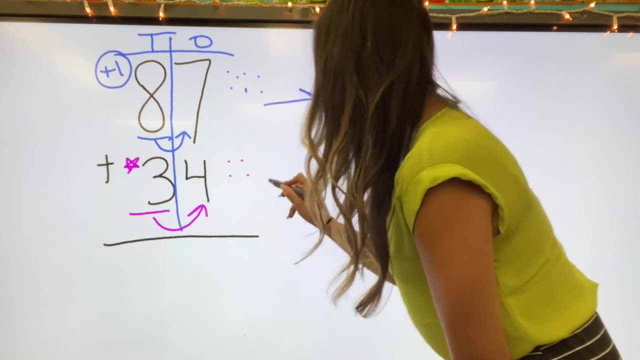 Five or greater, add one more. Four below, let it go. So four is less than five, so I'm gonna leave this three alone and bring it over here to 30.. So now that I've rounded both numbers, I'm ready to add. 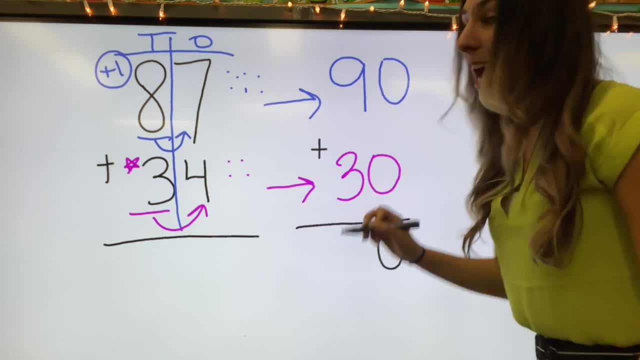 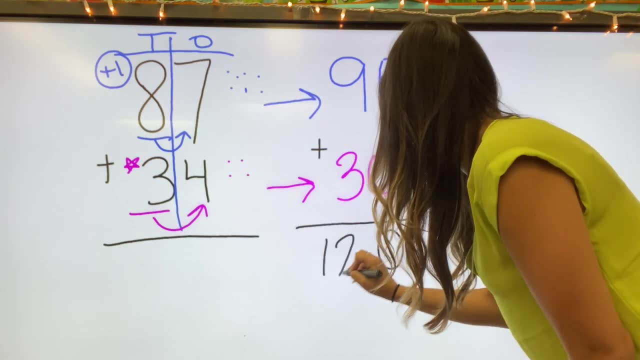 Zero plus zero equals zero. Nine plus three. I'm gonna put nine in my head, three on my fingers, Nine, ten, eleven, twelve. So my answer is 120.. So let's go back over our steps. So we're gonna go back over the steps. 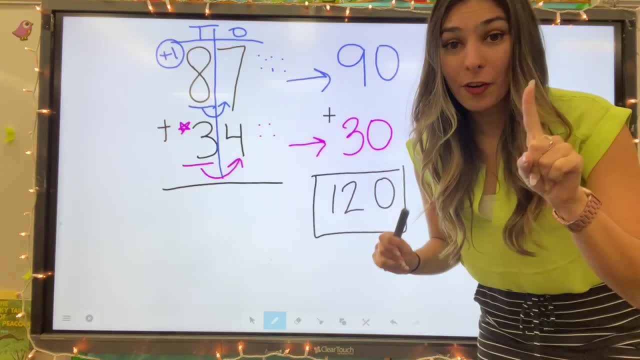 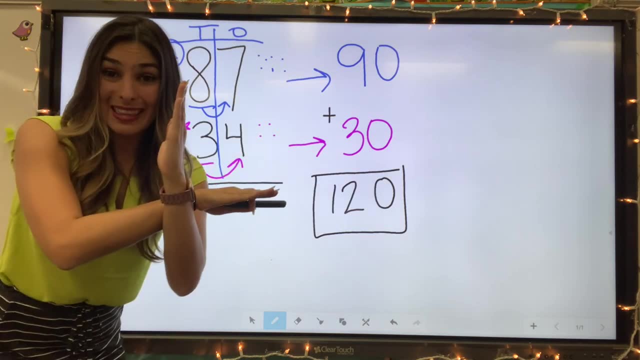 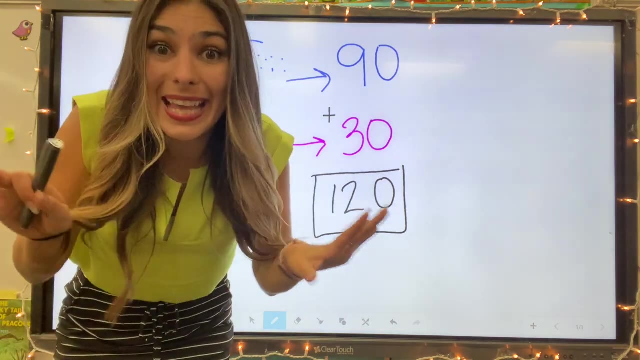 So my answer is 120.. So let's go back over our steps. First, we rounded each number. The 87 goes to 90 and 34 rounded to 30. We added them up and found the estimated sum is 120.. Now, when we estimate, it is not the exact number that this would add up to. 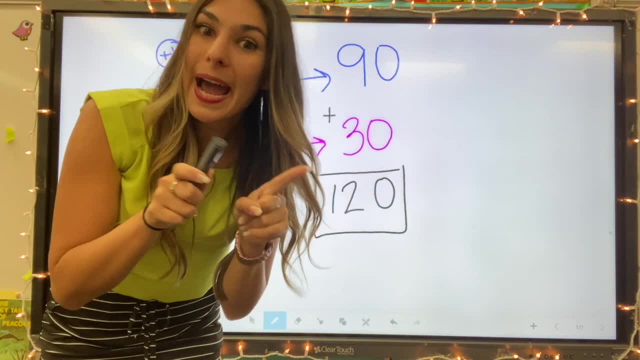 but it's okay because we're looking for the estimate We're looking for about how many. So let's actually add this up and see if we were close. We would add ones first. So 7,, 8,, 9,, 10,. 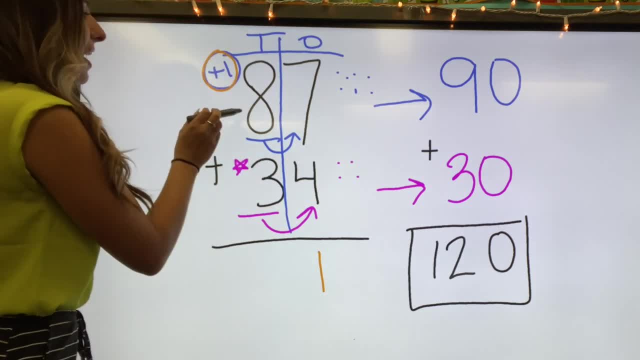 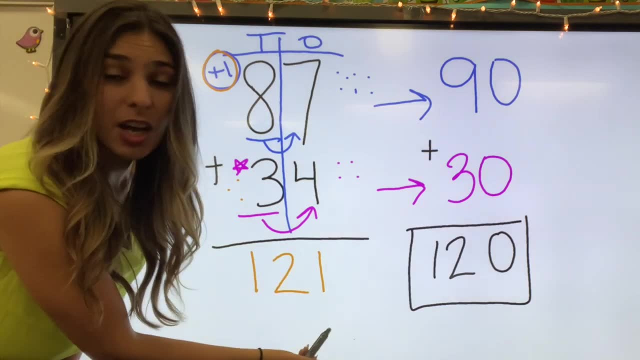 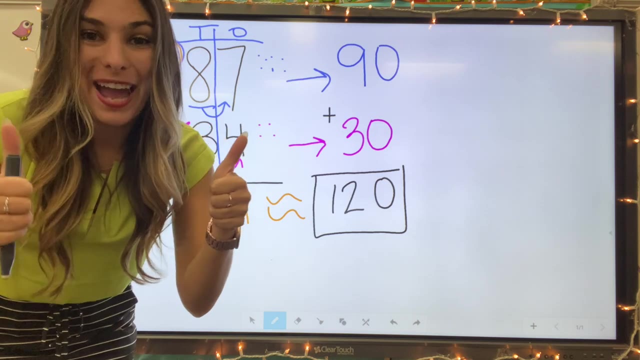 11.. Carry that one, We have 8,, 9,, 10,, 11,, 12.. So our real answer would be 121, which is about 120.. So our rounding and adding was correct, because this number is pretty dang close to this. 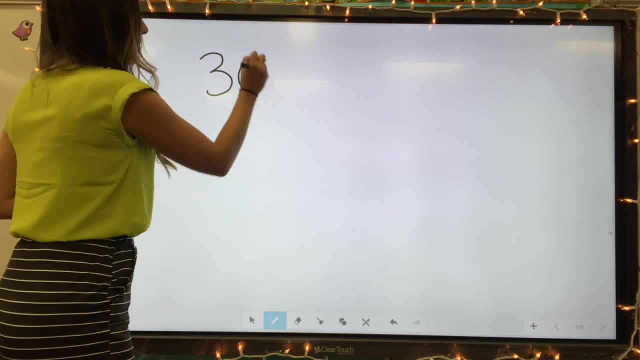 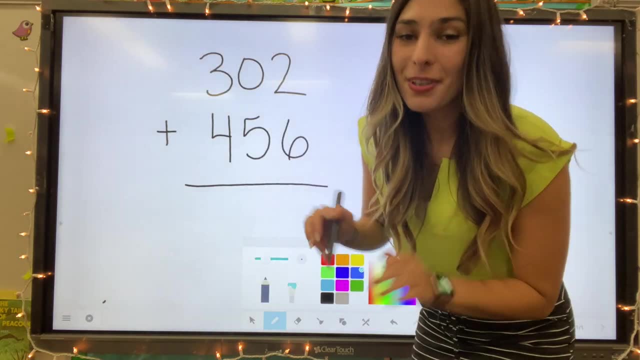 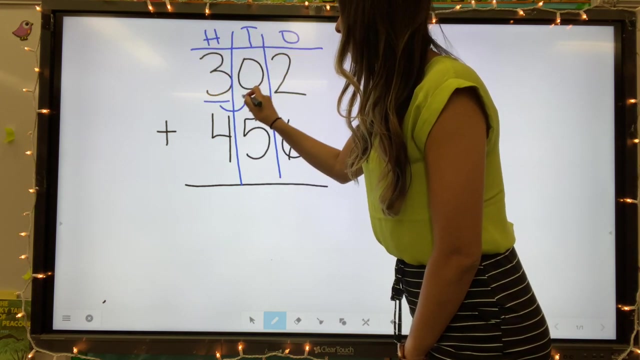 one. All right, let's do a bigger problem. Well, first thing I need to do is round each number. So to round. I'm going to follow my usual steps. My place is the 3.. I'm looking next door at that 0, and I'm asking myself: 5 or greater? 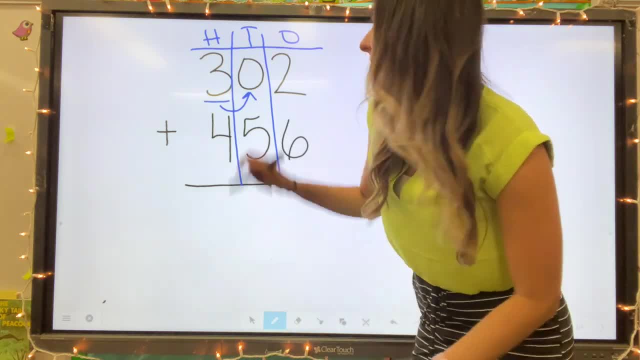 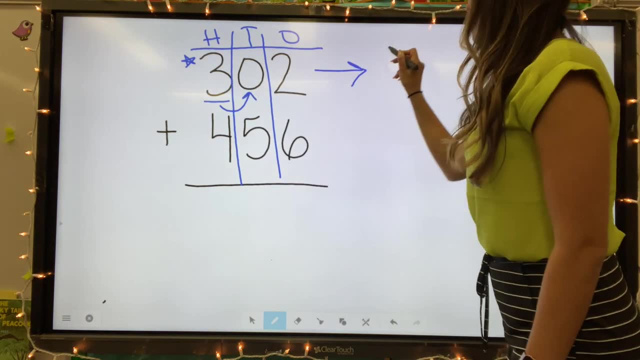 add one more 4 below. let it go That 0 is way less than 4, so we're going to keep this 3 and round 302 to 3.. Make that 100, 300.. Let's move on to our next number We have. 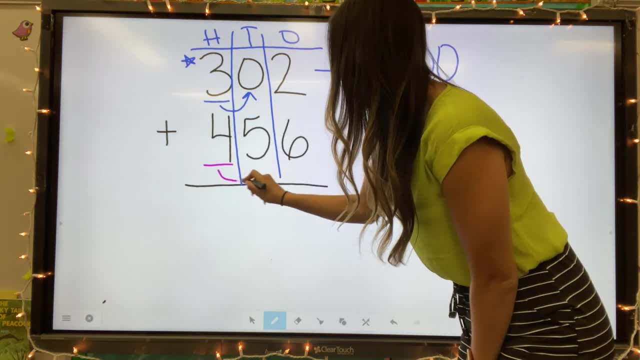 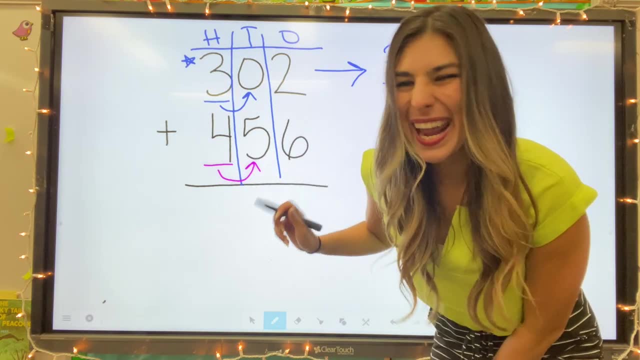 450.. My place is in the 100s. I look next door at that 5, and I ask myself: should we add one more or let it go? We're going to add one more. That 5 is too big. We're going to add one more to our 10,, so 4. 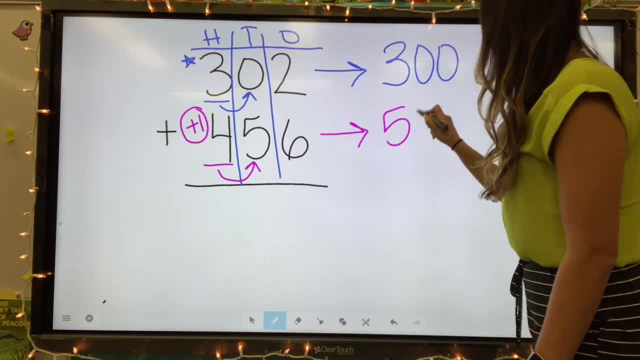 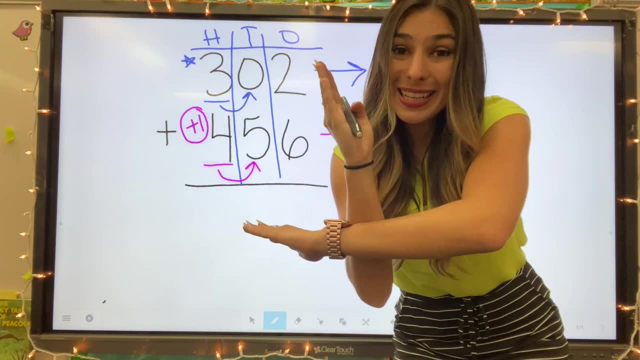 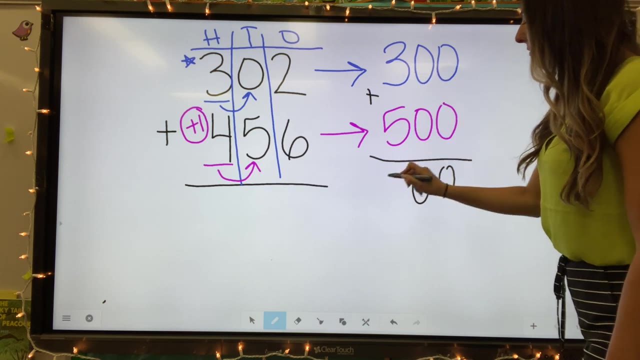 plus 1 equals 5.. We're going to make it 100.. So we rounded 456 to 500.. Now that we've rounded each number, we need to add them up. 0 plus 0 equals 0.. 0 plus 0 equals 0.. 3 plus 5 equals 8.. So our estimated number is 800.. So let's add this one. 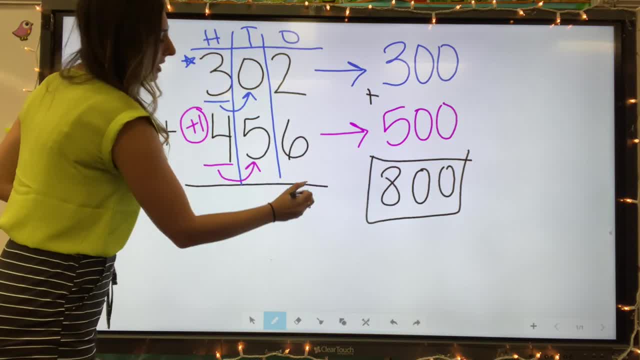 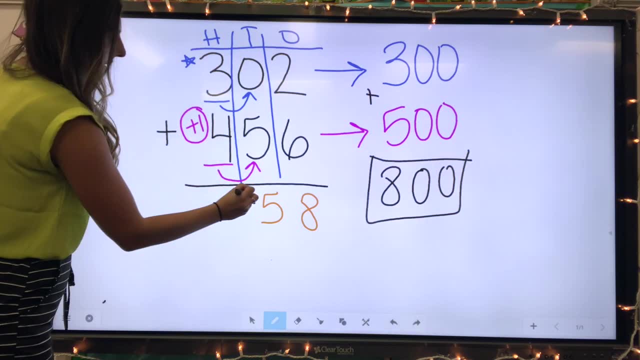 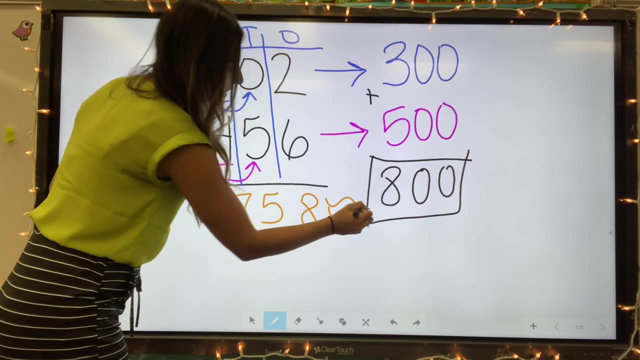 up and double check our work. Start with our 1s. We have 2 plus 6. That equals 8.. 0 plus 5 equals 5.. 3 plus 4 equals 7.. This added 1 goes for there, not for this. normal adding 758 is about 800.. We. 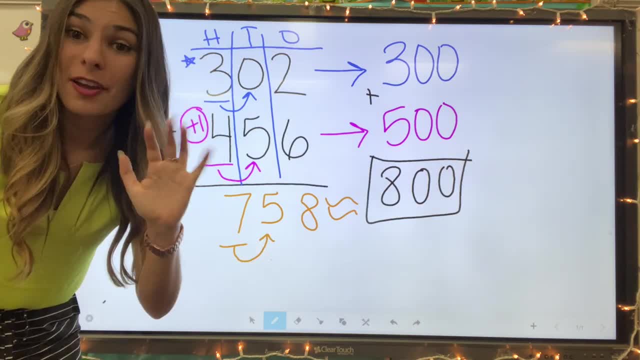 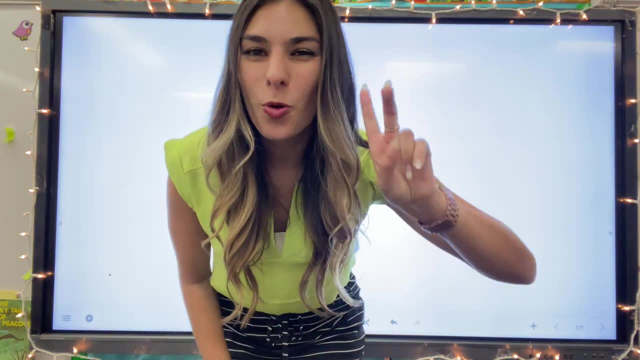 would round up Because that 5,, 5 or greater add one more. This is why we rounded to 800.. Okay, we're going to do two more problems with a little different way to round, So whichever one you like best. 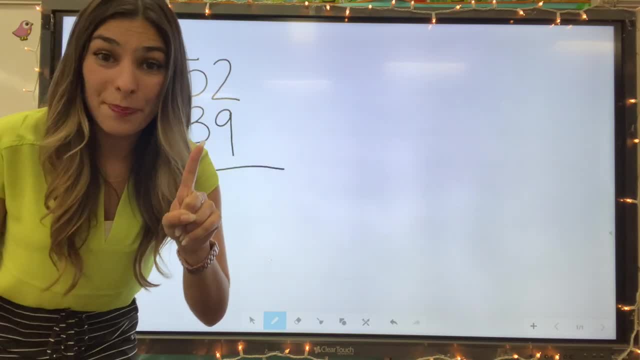 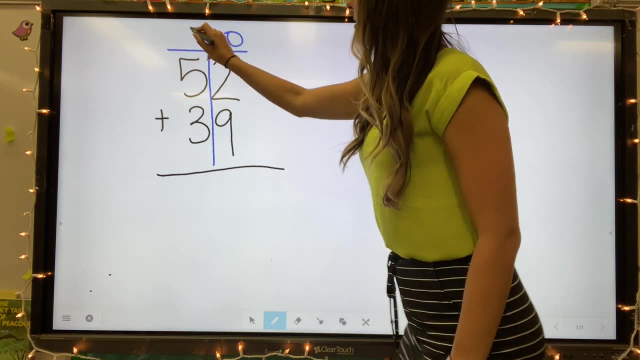 52,, 5,, 39.. Step one: I need to round each number, So I'm going to take 52, find my place. 1s and 10s. This first one is the 5.. I'm going to look next door at this, 2.. And with that, 2,. 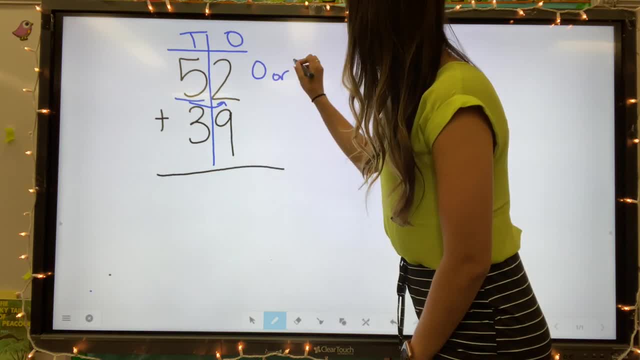 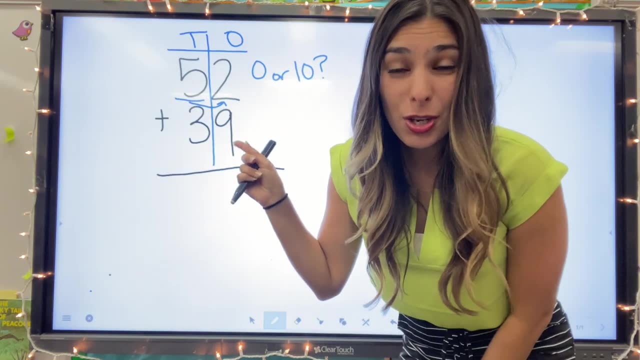 I'm going to ask myself: is it closer to 0, or 10?? So is that 2 closer to 0 or closer to 10.? THAT 2 IS WAY CLOSER TO 0.. SO WE'RE GOING TO ADD 0.. 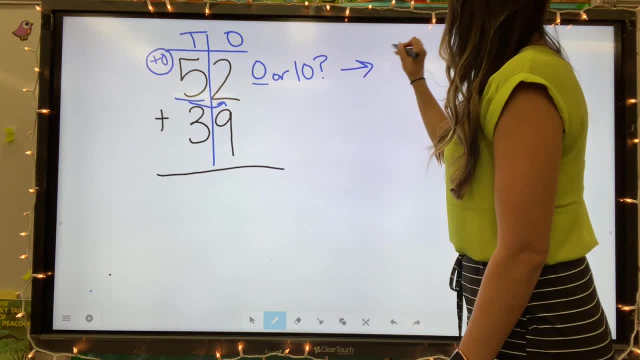 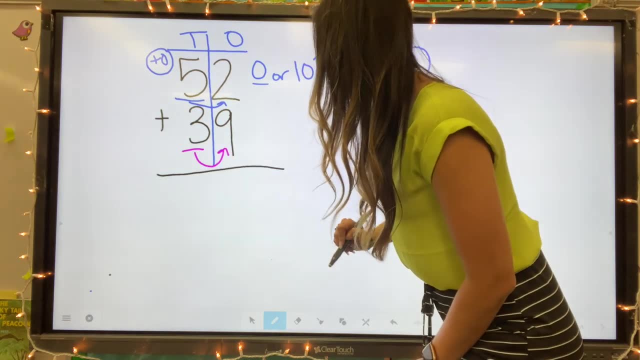 5 plus 0.. So we're going to come over here and round 52 to 50.. Next number, we have 39.. 3 is my place. I'm looking at that- 9.. And i'm going to ask myself: IS THAT 9 CLOSER TO ZERO? 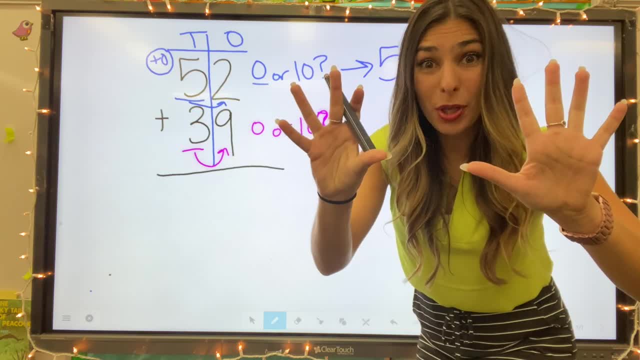 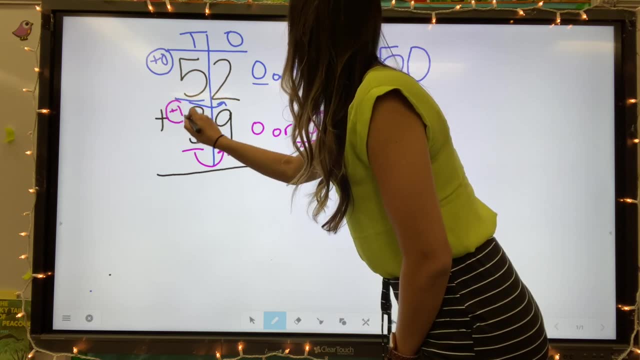 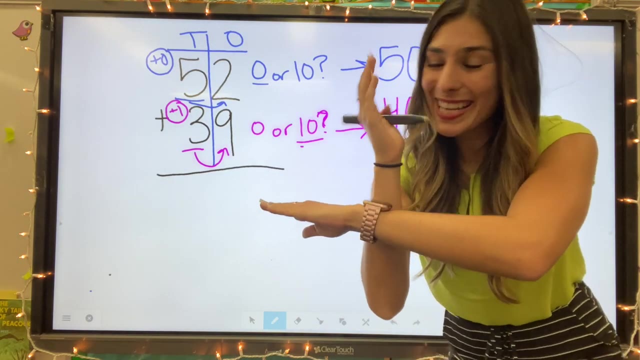 0 or 10?? Well, here's 9.. Only one more to get to 10.. It is way closer to 10.. So we're going to add 1.. 3 plus 1 equals 4.. So now that I've rounded my numbers, I'm ready to add. 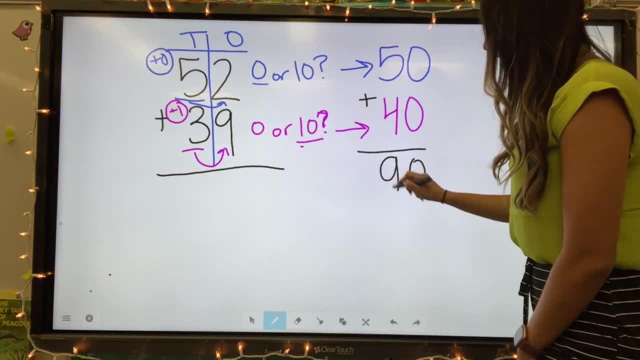 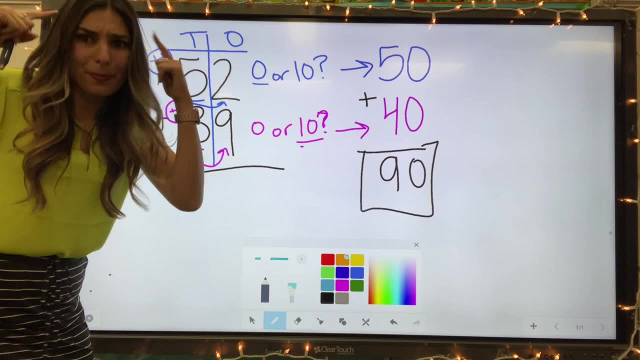 0 plus 0 equals 0.. 5 plus 4 equals 9.. Our estimated number is 90.. As always, let's double check our answer: 2 plus 9.. I'm going to put the biggest number in my head: 2 on my fingers, 9,. 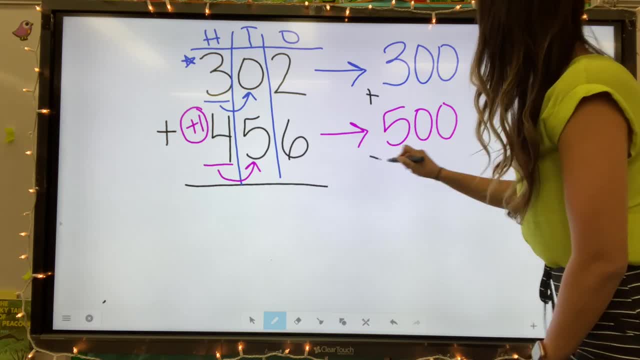 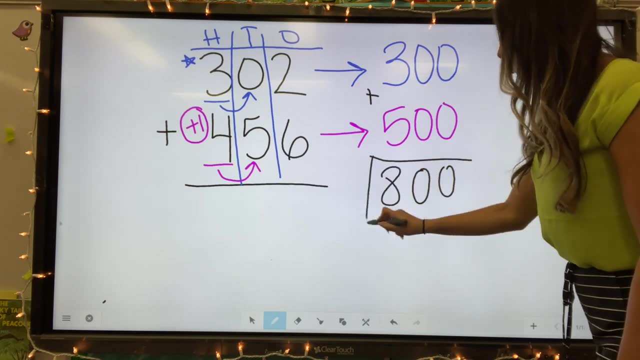 rounded each number. we need to add them up. Zero plus zero equals zero. Zero plus zero equals zero. Three plus five equals eight, So our estimated number is eight hundred. So let's add this one up and double check our work. Start with our. 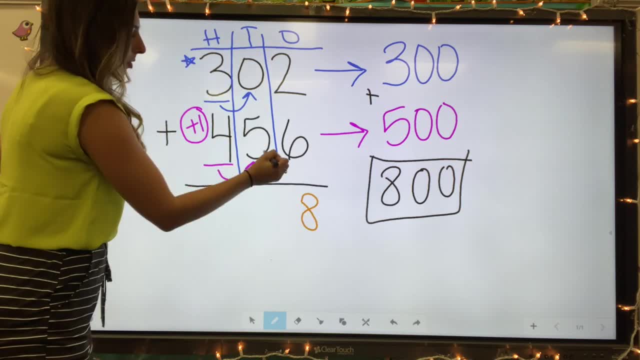 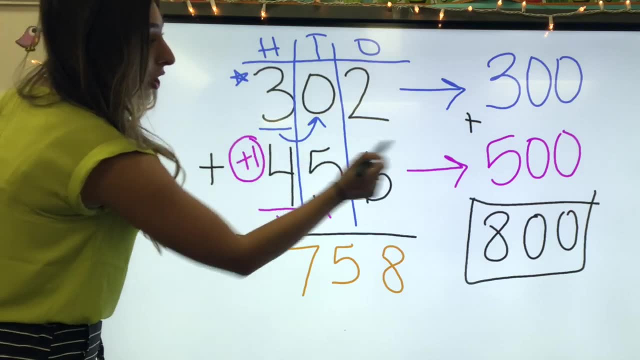 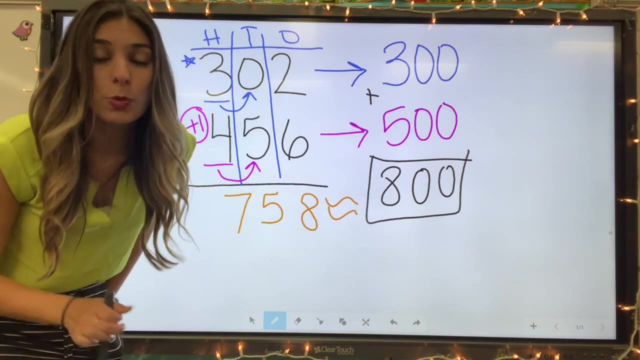 ones. We have: two plus six, That equals eight. Zero plus five equals five. Three plus four equals seven. This added one goes for there, not for this. normal adding 758 is about 800.. We would round up because that 5,, 5 or greater add one more. This is why we 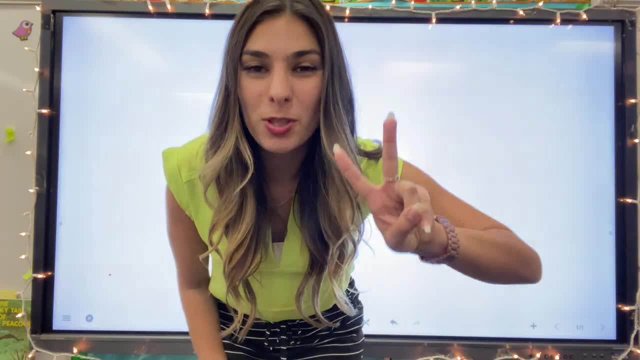 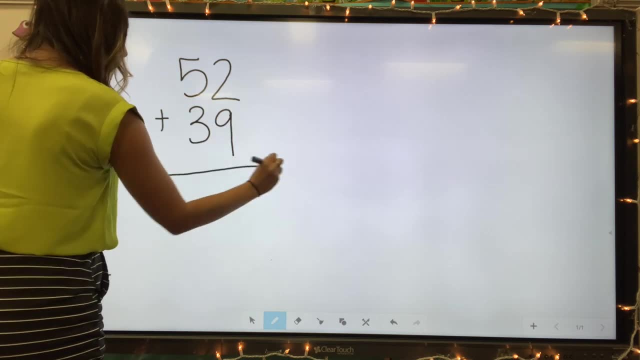 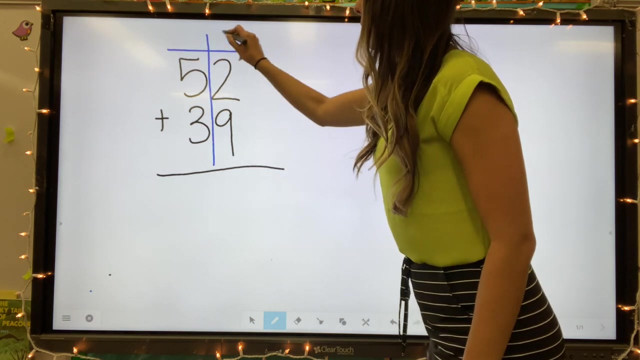 round it to 800.. Okay, we're going to do two more problems with a little different way to round, So whichever one you like best. Step one: I need to round each number, So I'm going to take 52,, find my place ones and tens. This first one is the five. I'm going to look next door at this two. 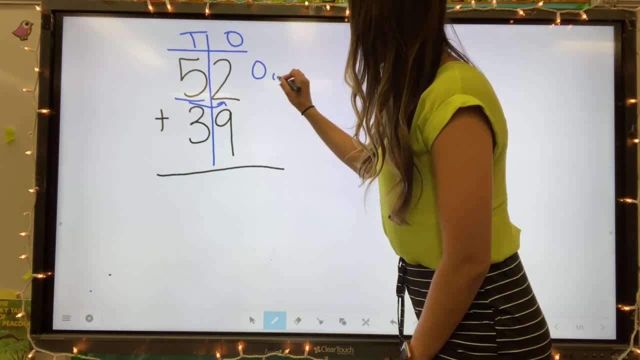 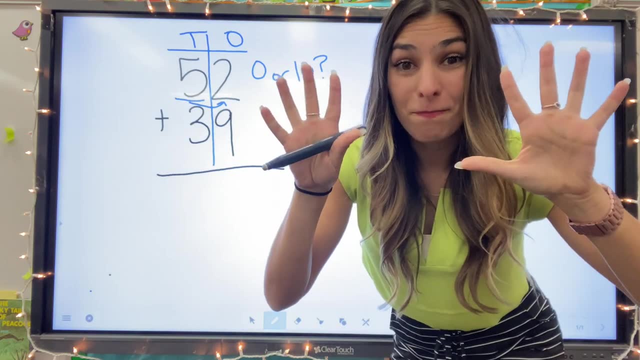 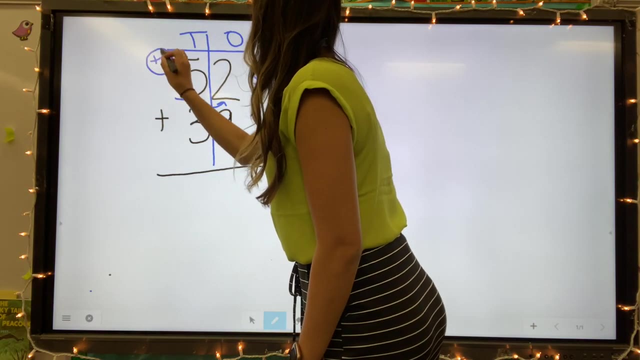 And with that two I'm going to ask myself: is it closer to zero or ten? So is that two closer to zero or closer to ten? That two is way closer to zero. So we're going to add zero, Five plus zero. So we're going to come over here and round. 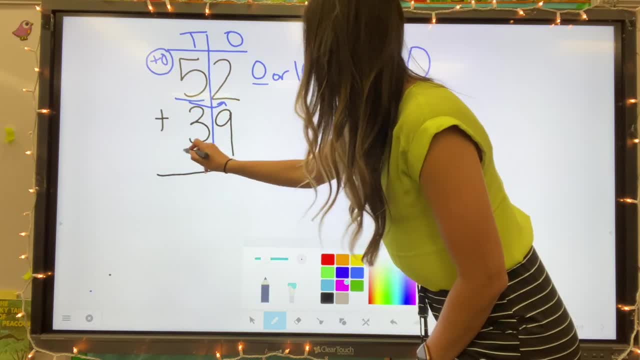 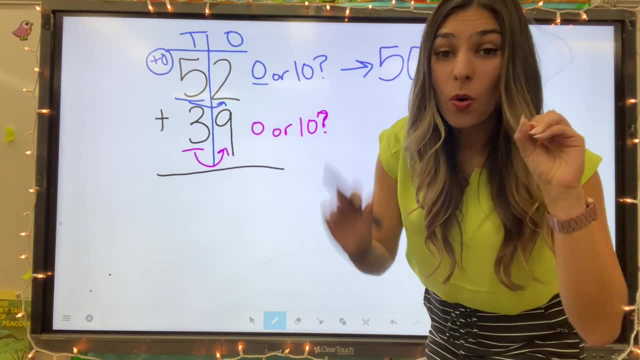 52 to 50.. Next number, we have 39.. Three is my place. I'm looking at that nine And I'm going to ask myself: is that nine closer to zero or ten? Well, here's nine. Only one more to get to ten. 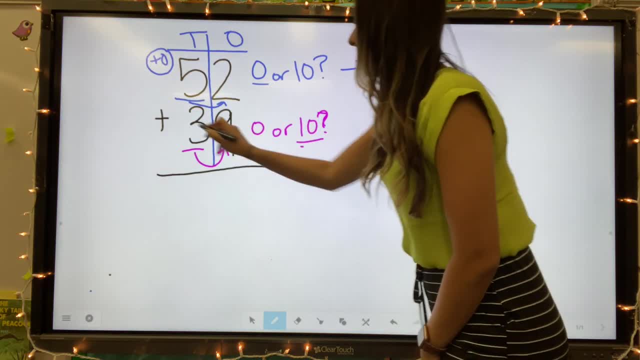 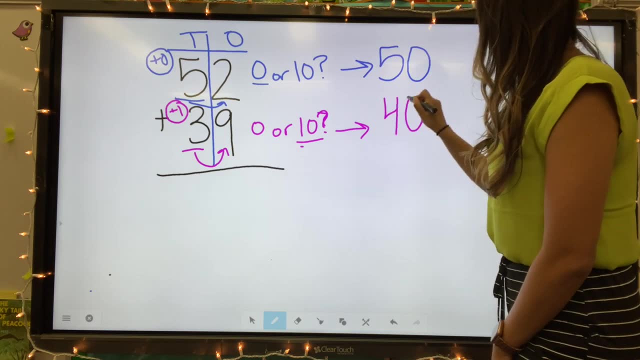 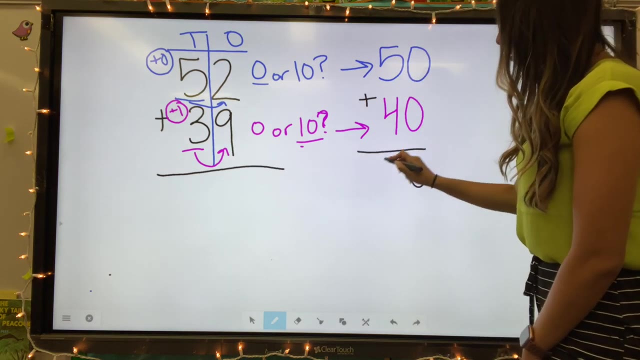 It is way closer to ten. So we're going to add one. Three plus one equals four. So now that I've rounded my numbers, I'm ready to add Zero plus zero. Zero equals zero. Five plus four equals nine. Our estimated number is 90.. As always, let's double. 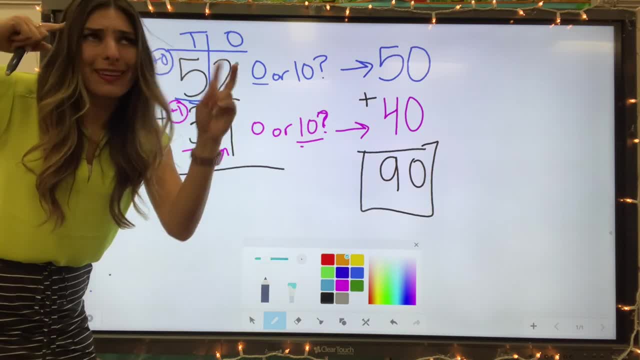 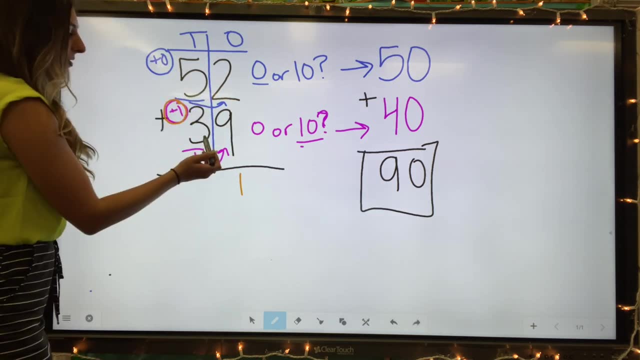 check our answer: Two plus nine- I'm going to put the biggest number in my head, Two on my fingers- Nine, ten, eleven, Eleven, And here's that one that we carry. Five plus three equals eight, plus one equals nine. So we had 91 and we rounded it down to 90. So this: 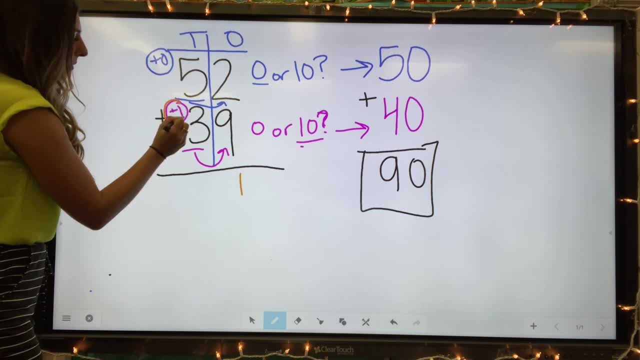 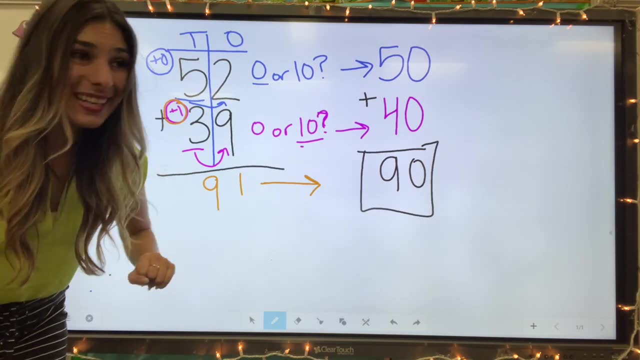 10,, 11,, 11.. And here's that 1 that we carry: 5 plus 3 equals 8, plus 1 equals 9.. So we had 91 and we rounded it down to 90. So this is accurate. All right, let's do the same way with the bigger. 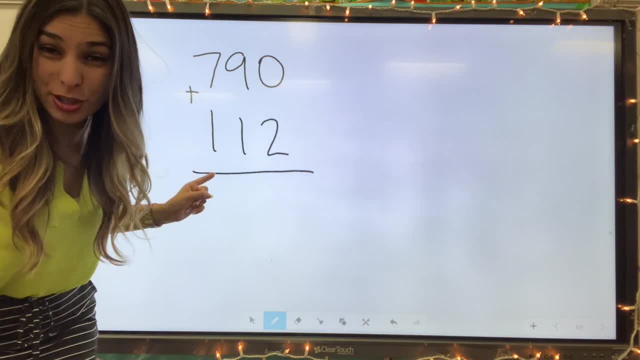 number. Okay, so if I have 790 plus 112, first thing we need to do round each number. So, just like we always would to round, I'm going to round each number. So I'm going to round each number. 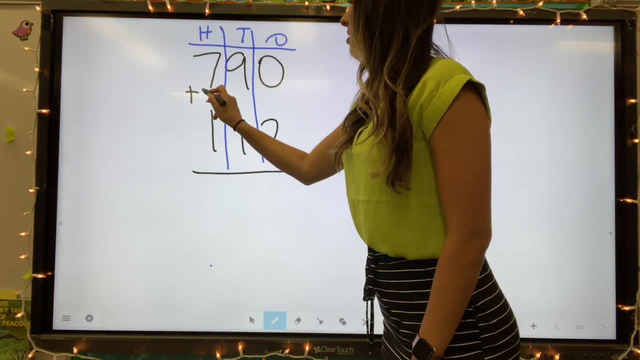 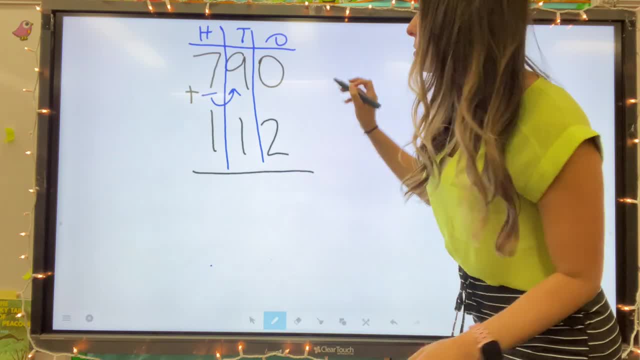 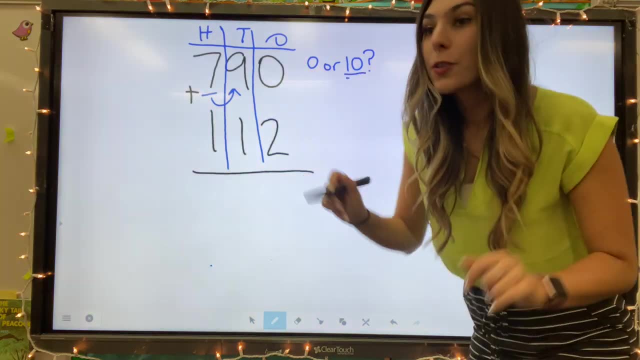 And I'm going to ask myself this time: is that 9 closer to 0 or 10?? Show me 9.. That 10's right there. So because it's closer to 10, I'm going to add a 1 here. 7 plus 1 equals 8.. 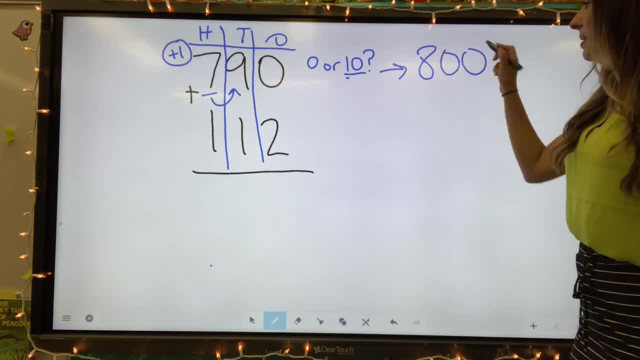 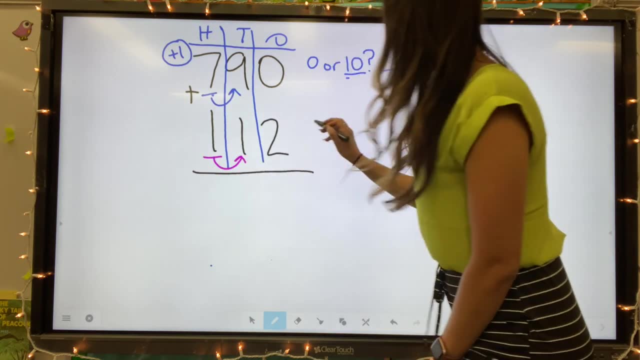 So I'm going to do 8 and make it a 100, because we are running to the nearest 100.. Next number: 100th place. Look next door at that. 1.. Ask myself, is that 1 closer to 0 or a 10?? 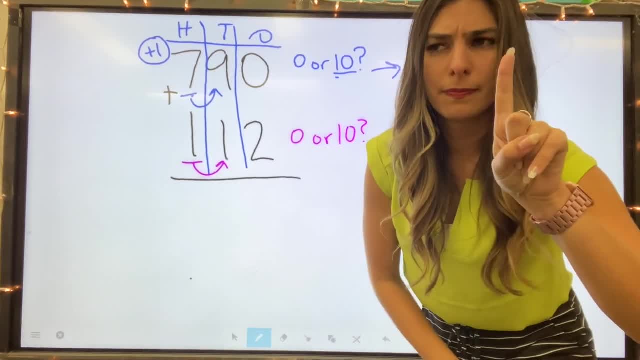 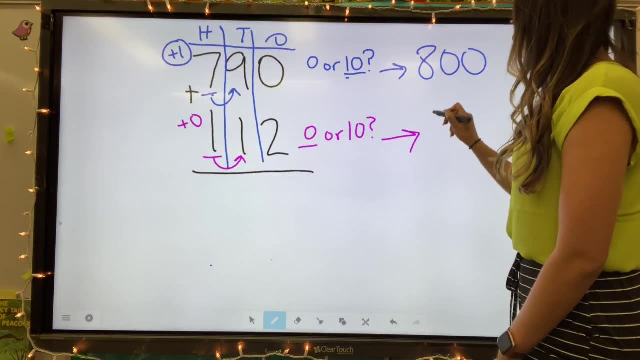 Is that 1 closer to 0 or 10?? Way closer to 0.. Because it's closer to 0, I'm going to add 0. And 1 plus 0 equals 1.. So I'm going to keep that 1 here. make it a 100, because we're running to. 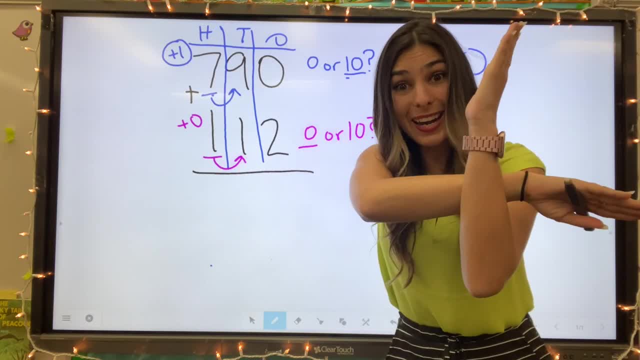 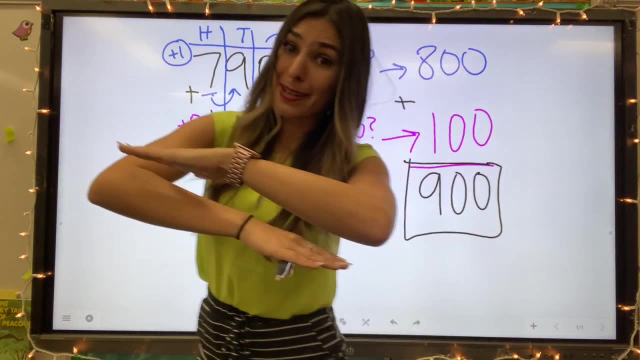 the nearest 100.. And now that we've rounded our numbers, we're ready to add: 0 plus 0 equals 0.. 0 plus 0 equals 0.. 8 plus 1 equals 9.. So our estimated sum is 900.. Let's double check our work though. 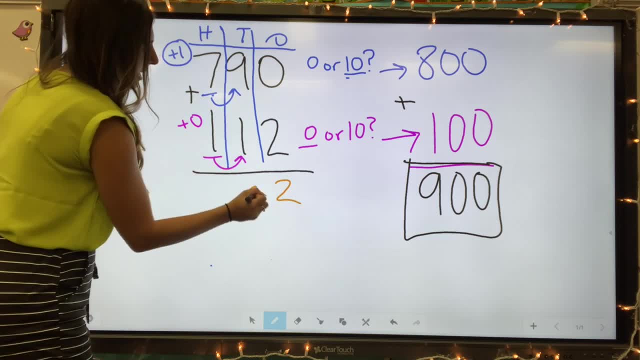 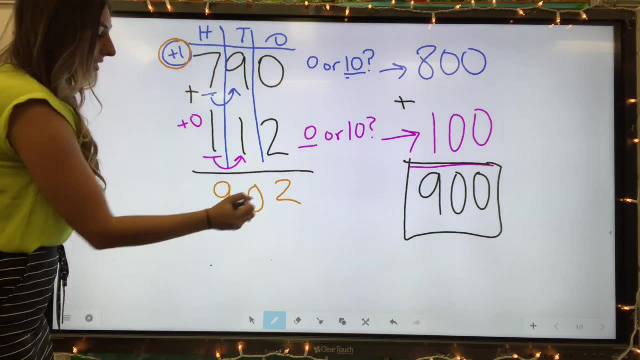 0 plus 2 equals 2.. 9 plus 1 equals 10.. I'm going to carry that 1. that's up here. 7 plus 1 equals 8. Plus 1 equals 9. 902.. Except we rounded to 900.. We are all good. 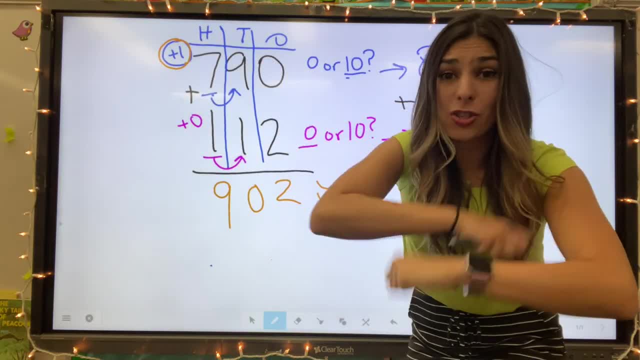 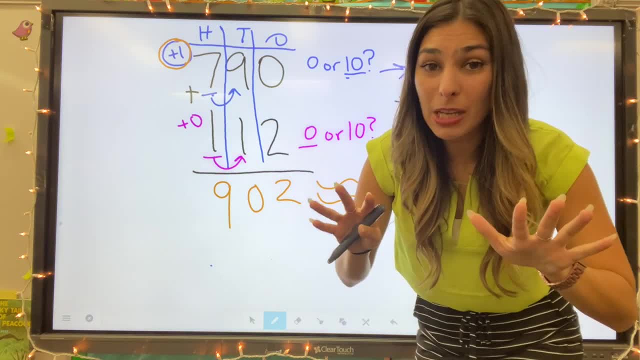 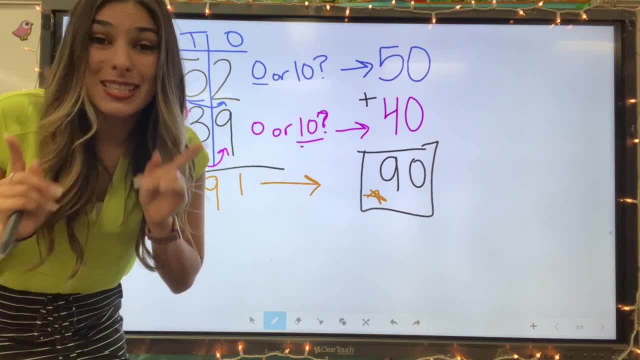 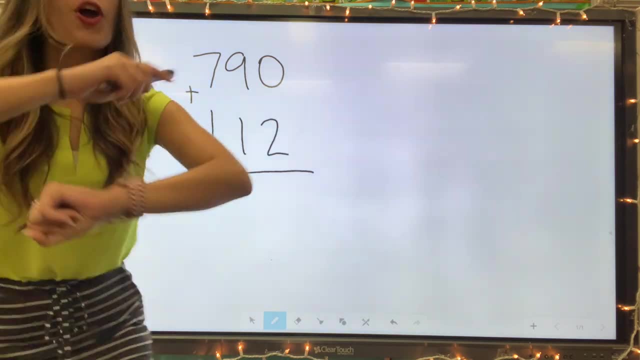 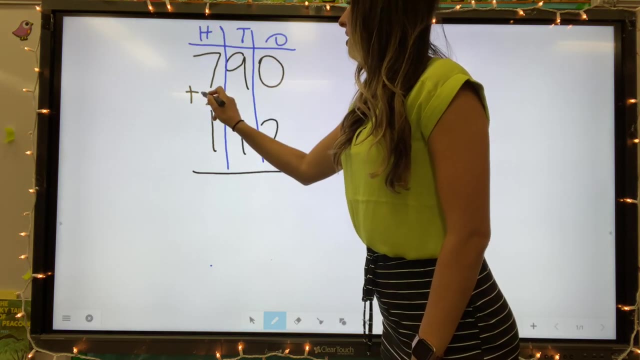 is accurate. All right, let's do the same way with the bigger number. Okay, so if I have 190 plus 112, first thing we need to do round each number. So, just like we always would to round, I'm going to find my place. I'm going to put the nearest hundred, looking next door at that nine. 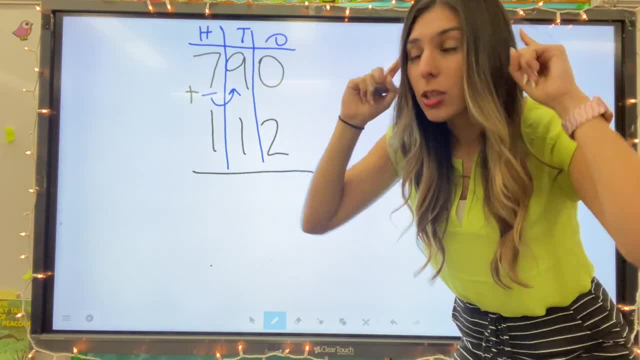 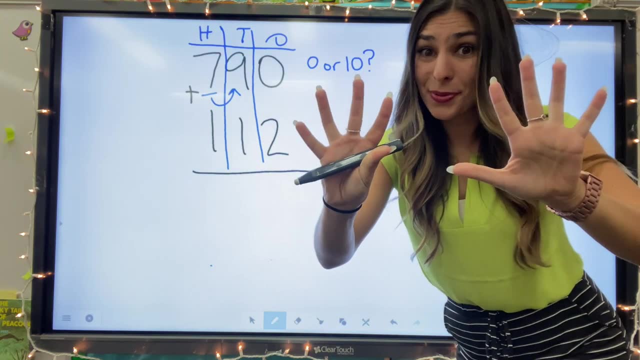 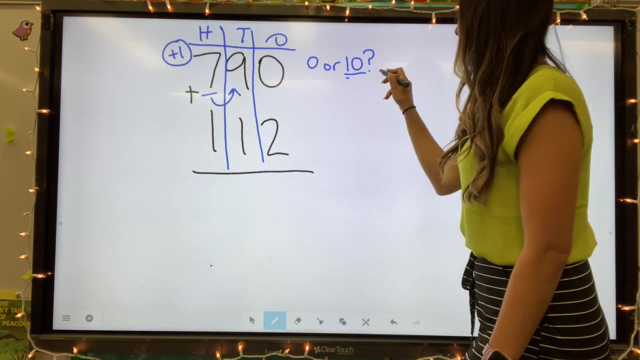 And I'm going to ask myself this time: is that nine closer to zero or ten? Show me nine, That ten's right there. So, because it's closer to ten, I'm going to add a one here. Seven plus one equals eight. So I'm going to do eight and make it a hundred, because we are running to the nearest. 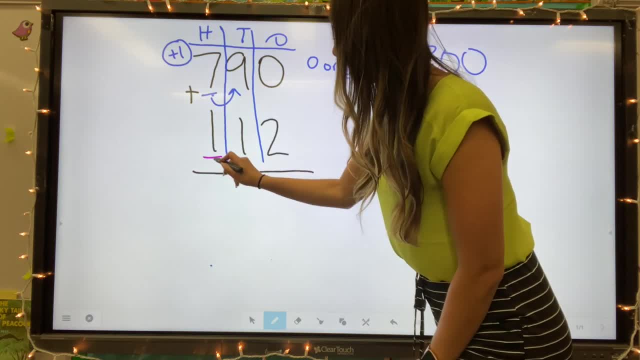 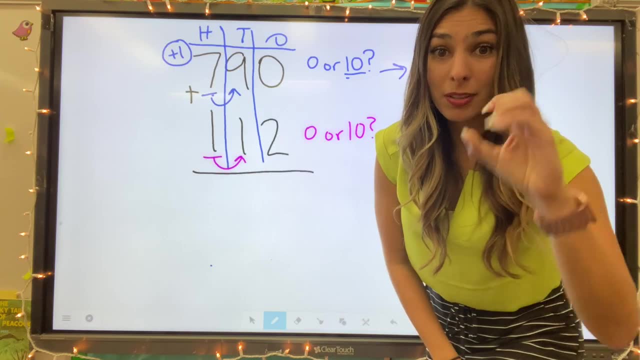 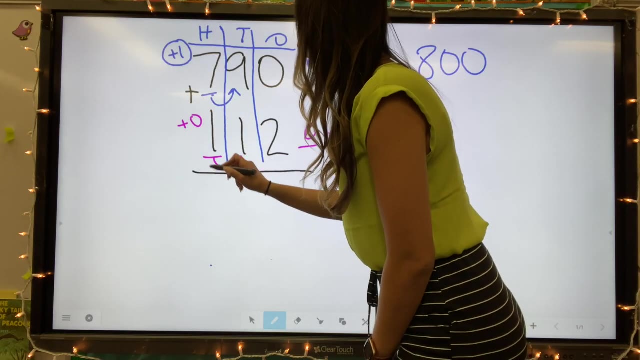 hundred. Next number, hundreds place. Look next door at that one. Ask myself: is that one closer to zero or a ten? Is that one closer to zero or ten Way closer to zero? Because it's closer to zero, I'm going to add zero, And one plus zero equals one, So I'm going to keep that one here. 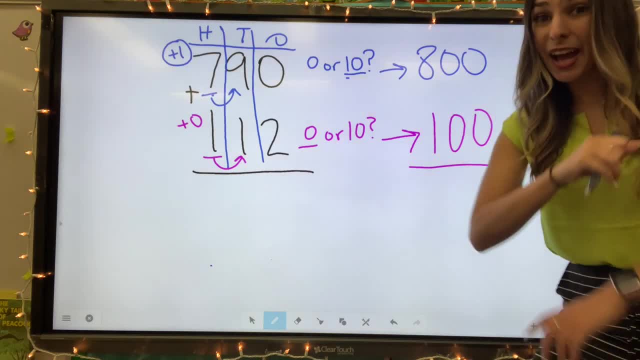 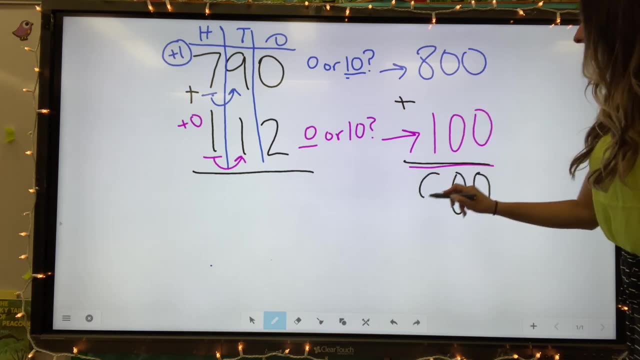 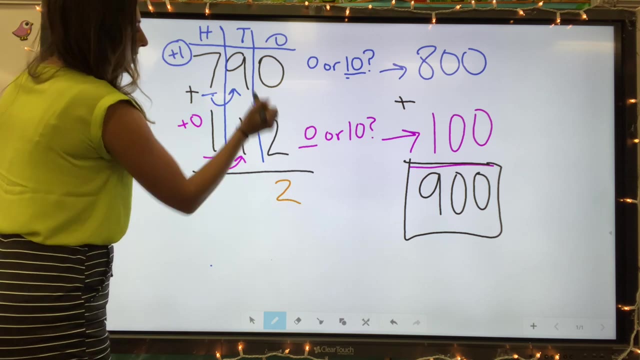 make it a hundred, because we're running to the nearest hundred, And now that we've rounded our numbers, we're ready to add. Zero plus zero equals zero. Zero plus zero equals zero. Eight plus one equals nine, So our estimated sum is nine hundred. Let's double check our work, though: Zero plus two equals two. Nine plus one. 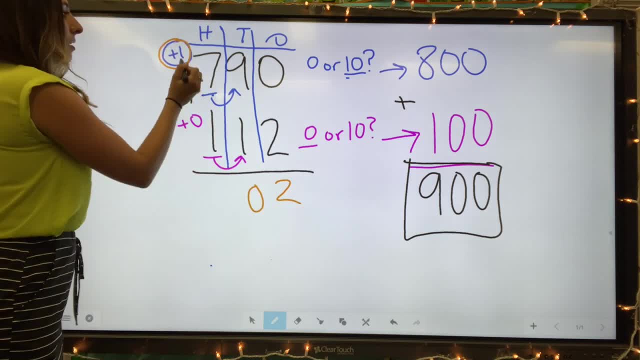 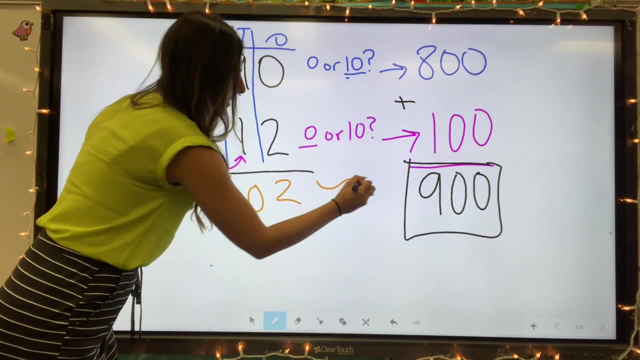 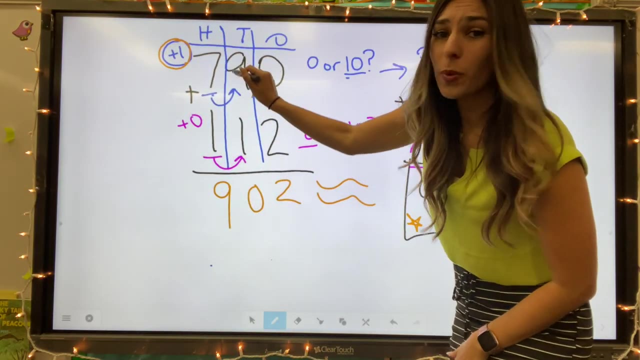 equals ten. I'm going to carry that one that's up here. Seven plus one equals eight. Plus one equals nine. Nine hundred and two, except we rounded to nine hundred. We are all good. So just to go over our work. First we rounded each number, added the rounded. 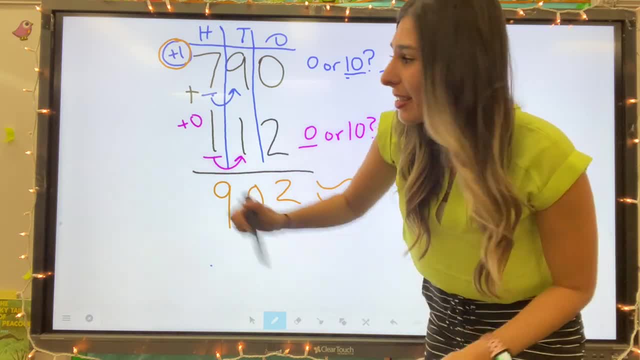 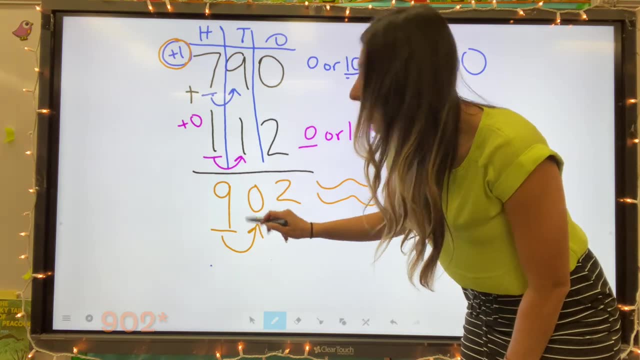 numbers and found the estimated sum, And we double checked that by adding up our original addition problem, And if we took nine hundred and rounded it to the nearest hundred, we would have gotten nine hundred. That's how we know that we are correct. All right, guys. so thank you for rounding. 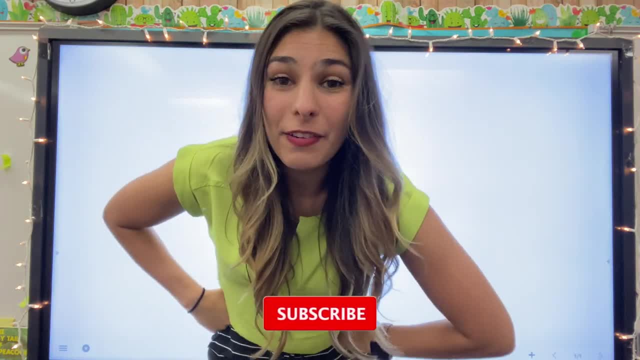 to estimate the sum with addition problems. If you liked this video or found it helpful, please give a big thumbs up. subscribe to the channel if you haven't already, and I'll see you guys in the next one. Bye, friends.